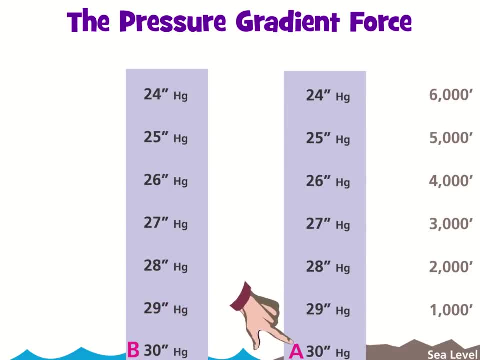 In other words, if each of these columns were resting on a scale, they would weigh the same. Now we know that atmospheric pressure decreases approximately one inch of mercury for every thousandth. Therefore, at 5,000 feet, in both columns of air, the pressure at positions 1 and 2 is 25 inches of mercury. 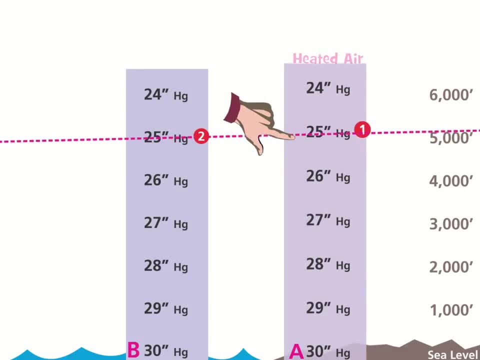 Now let's heat up the air in column A. Heated air expands, so the air in column A expands vertically by some small amount, As it does. watch what happens to the level where the air's pressure is 25 inches of mercury in that column. 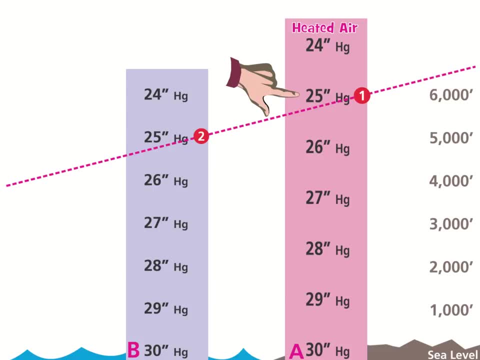 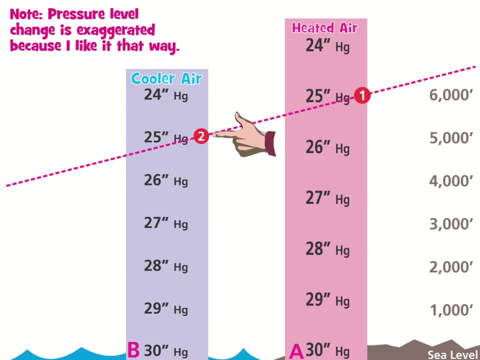 We can now say that uneven heating of air caused all the pressure levels in the vicinity of 25 inches of mercury to slope downward to the left slightly. As we know, if we move closer to sea level, the pressure increases. If we move upward away from sea level, the pressure increases. 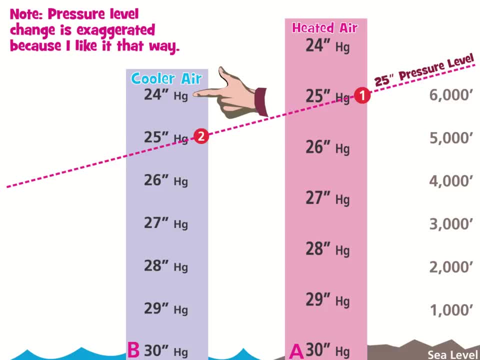 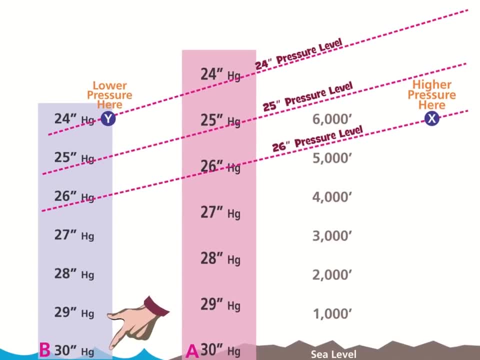 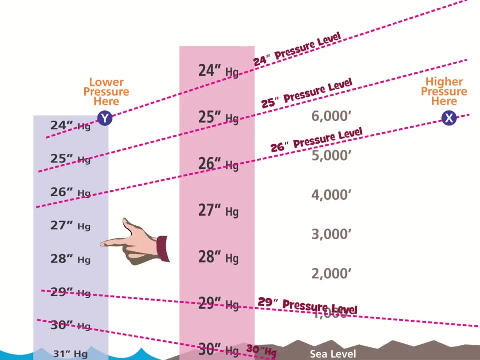 a cooler ocean. At sea level under column B, the cooler air produces a pressure of 31 inches of mercury. This difference in temperature produces slightly closer or compressed pressure levels at position 3 and expanded pressure levels at position 4.. Looking closely at position 3,, 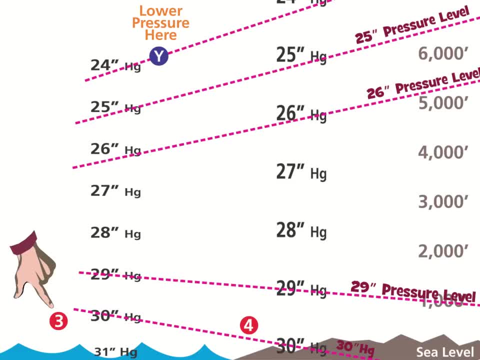 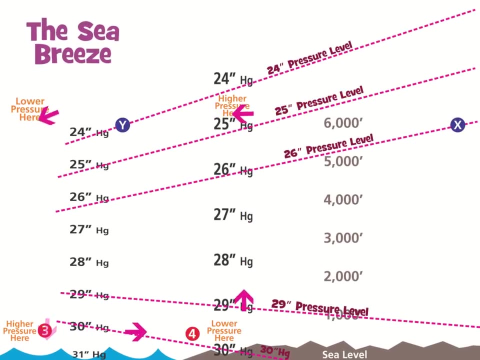 would a parcel of air at this position move right or left? Well, clearly it would move to the right, toward position 4, which is at a lower pressure, And this sets up the traditional closed-cell circulation known as a sea breeze, that typically occurs during daylight hours, Of course, at night, 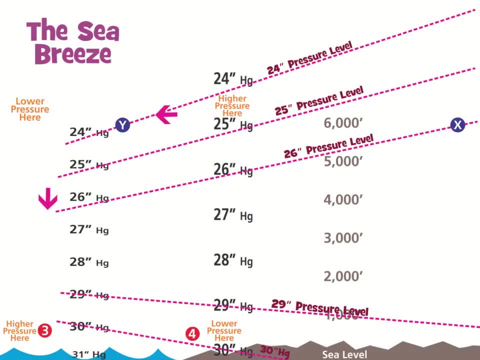 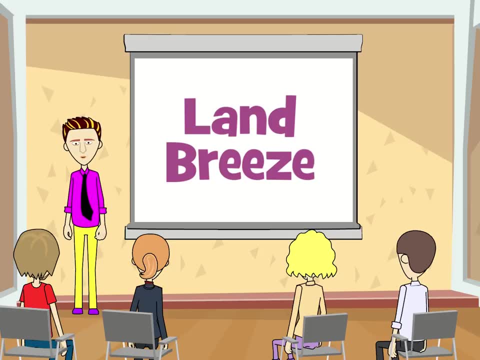 the land cools quickly, while the ocean retains much of the heat it absorbed during the day. Therefore, air and land switch temperature profiles, with the land being cooler than the ocean and the circulation reverses, becoming a land breeze instead. Well, congratulations, You now know the basics of how wind is generated by tilting. 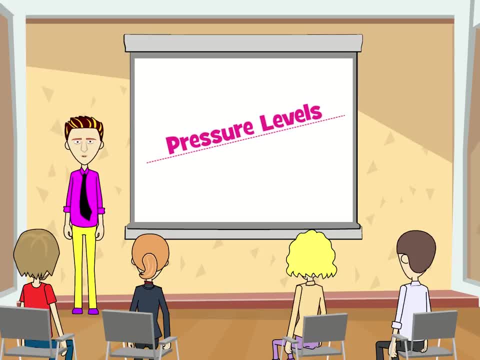 pressure levels, In other words, when pressure levels expand or compress in the vertical direction as a result of the heating or cooling of large masses of air. Believe it or not, if you can understand this basic principle of the pressure gradient force, you can easily 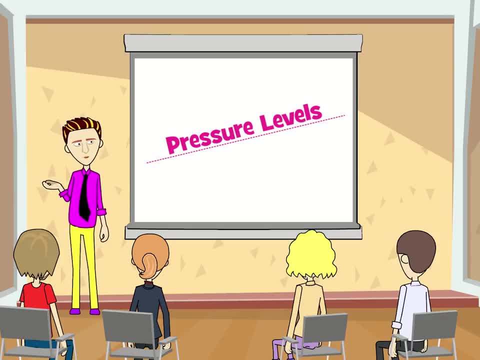 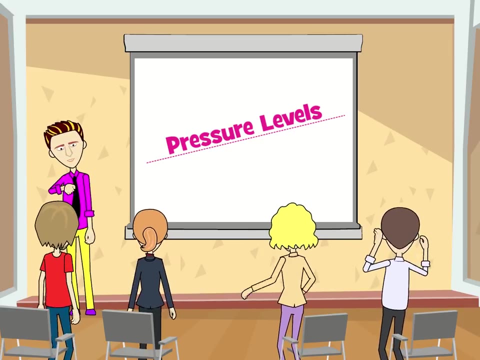 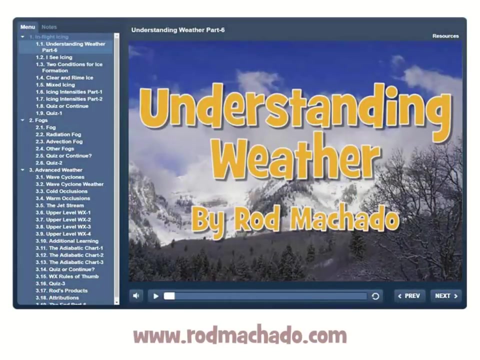 understand how the low-altitude and high-altitude jet streams form, to name a few. So onward and upward and, as they say, south of the border, hasta la bye-bye. Greetings folks. Rod Machado here If you would like to learn more about meteorology and 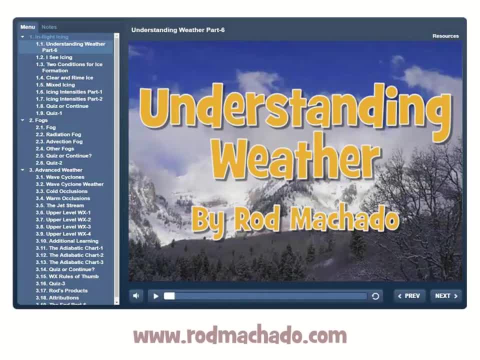 understanding weather as it applies to flying an airplane, then please consider purchasing my five-and-a-half-hour course on understanding weather For pilots. you'll find this course to be very helpful in understanding some of the very complex phenomena that occur in meteorology. This course can be found at my website at rodmachadocom.